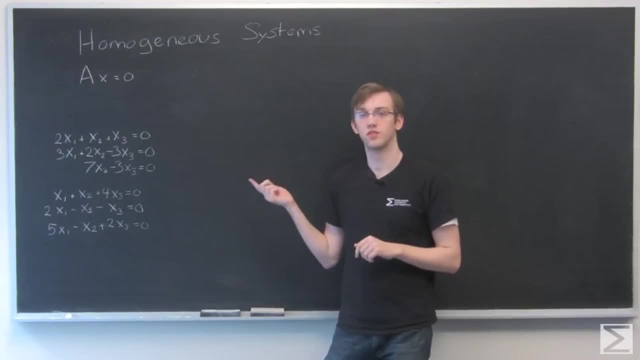 or it can have infinitely many. For a homogeneous system, it can have a number of solutions, but it can also be a problem. So if you have a homogeneous system, the that first option is ruled out, where there's no solutions, because every homogeneous system at least has one solution. 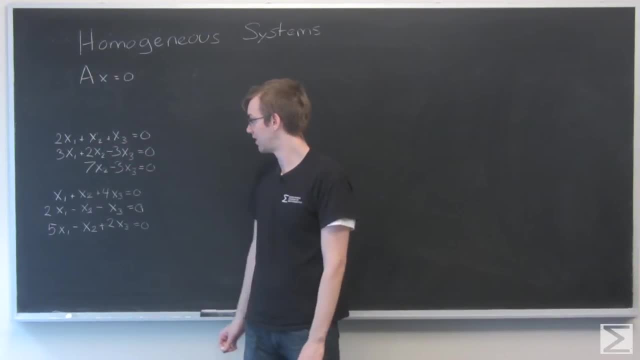 which is the trivial solution, which is where x1,, x2,, x3 are all equal to 0. And so the question basically becomes: is there a, is there a solution beyond the trivial solution, where everything is equal to 1? So for these two examples, one of them's going to be trivial, one of them's going to be 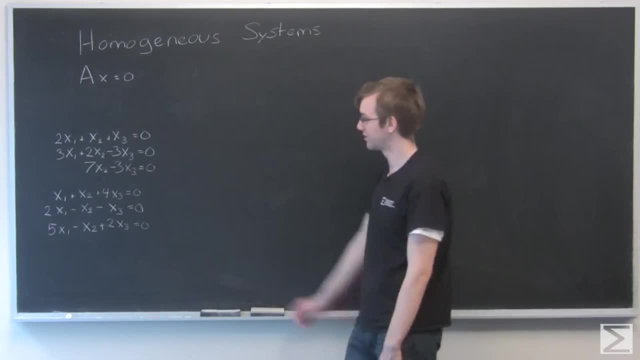 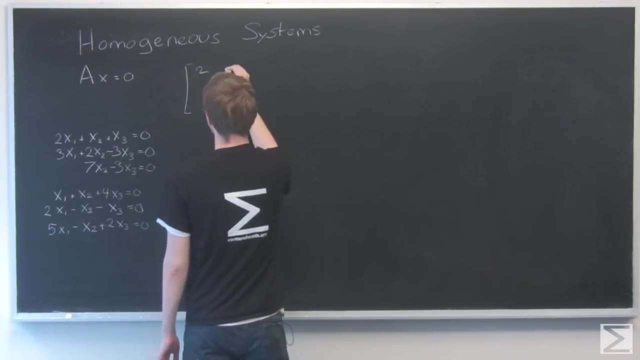 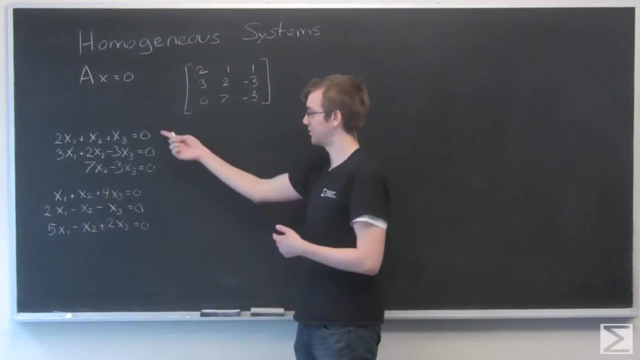 non-trivial And we're going to solve them just to see what it looks like. So let's write this as a coefficient matrix. So you might be asking yourself, why didn't you include those zeros? Well, if you think about the elementary row operations, that 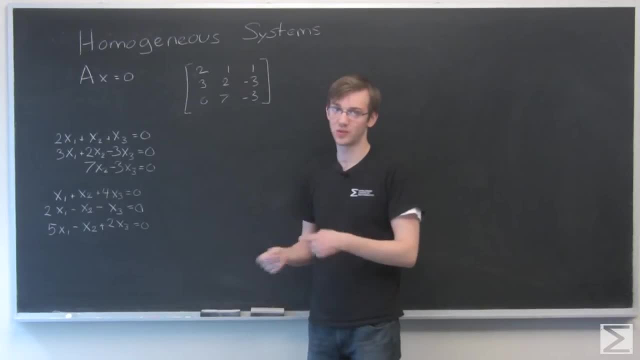 we do on the matrix. we can multiply by a constant, we can swap rows, we can add rows to each other. Those zeros are never going to change. They're just going to stay as a row of zeros through the whole thing. So if I'm working with a homogenous system, I don't 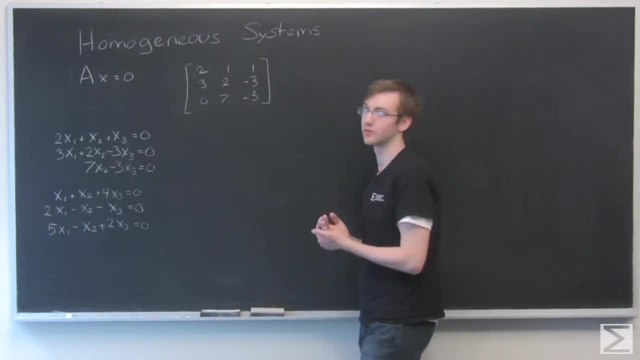 have to write that final row. I can just leave it off and remember that they're all equal to zero and that this isn't my solution, that my solutions are just all zero and they're not included. So I can just go about solving this. 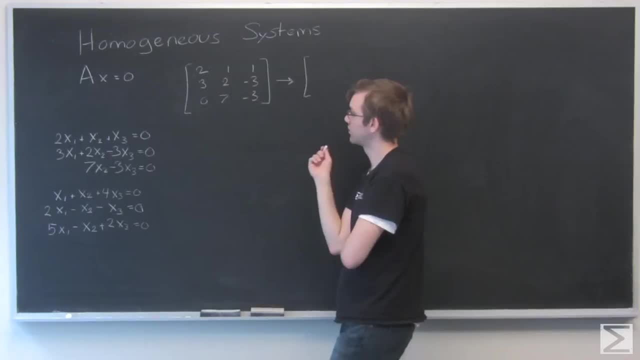 First thing I'm going to do, I'm going to subtract the first row from the second row. That won't get rid of it, but that'll give me a 1.. 3 minus 2 is 1.. 2 minus 1 is 1.. 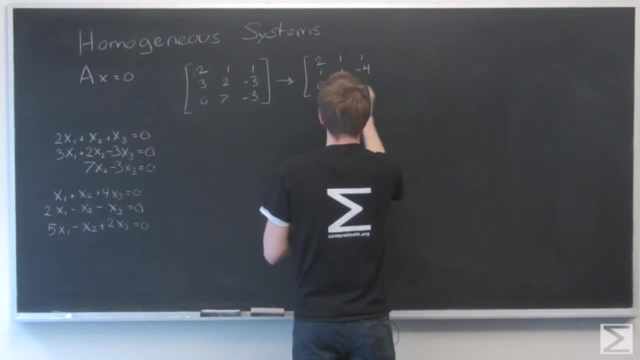 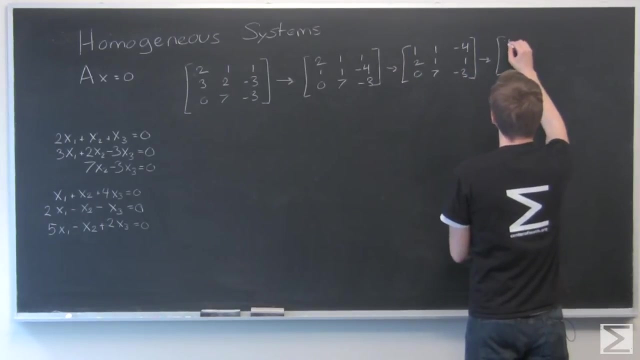 Minus 3 minus 1 is minus 4.. Now I'm going to swap and put that row with a leading one at the top, And now I'm going to go 2 minus 2 times the first row, 0.. 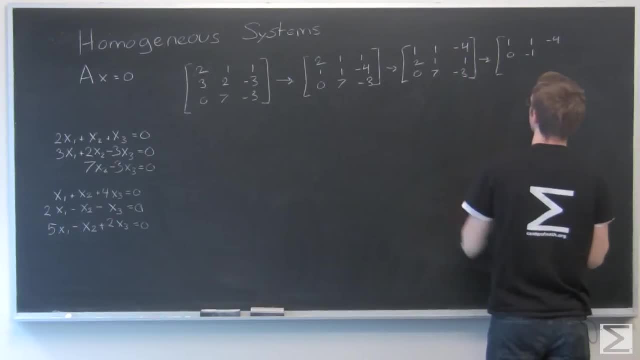 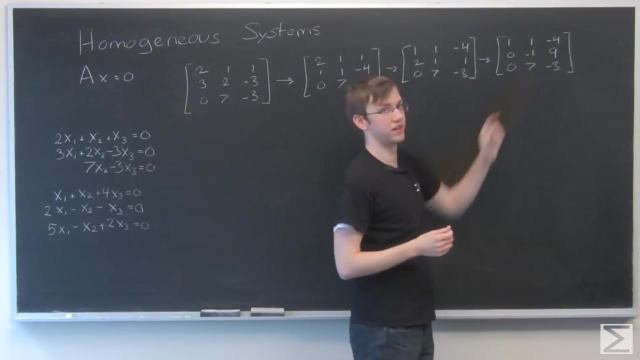 1 minus 2 is minus 1.. 1 minus 2 times minus 4.. 1 minus minus 8.. 1 plus 8 is 9. And 0, 7 minus 3.. OK, I'm going to multiply this by negative 1, real quick. 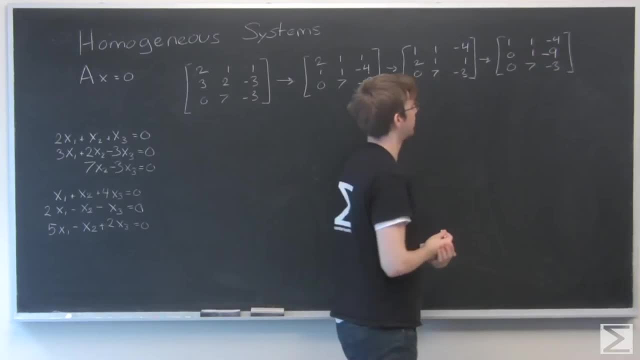 And now I'm going to use this 1 to get rid of that 7.. So that's 7 minus 7 times this row. Let me write 1, 1 minus 4.. 0, 1 minus 9.. 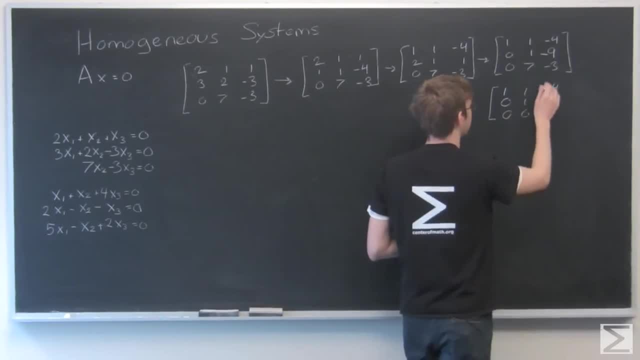 0.. And that's minus 3 times 7 times negative 9.. And that's minus 3 times 7 times negative 9.. It's minus 9.. And now I'm going to get rid of this 1 to get rid of that. 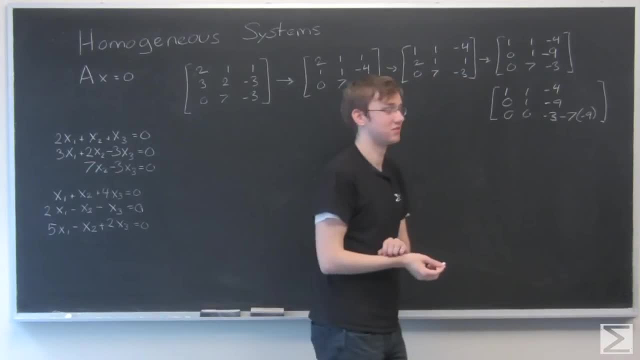 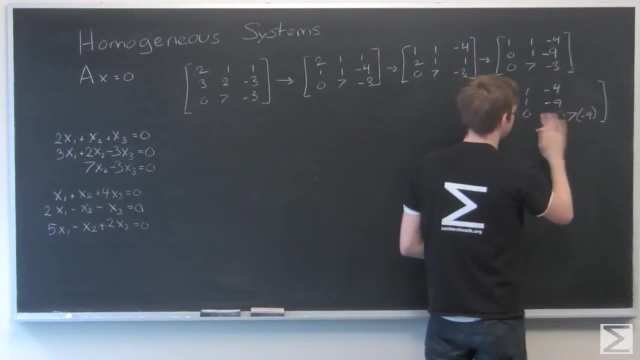 7. I'm not even going to solve that out or write down what that number is, because that's the last number I have in this row and I know whatever it is, I can just divide it by itself and I'll eventually get a 1 right there without affecting anything else. 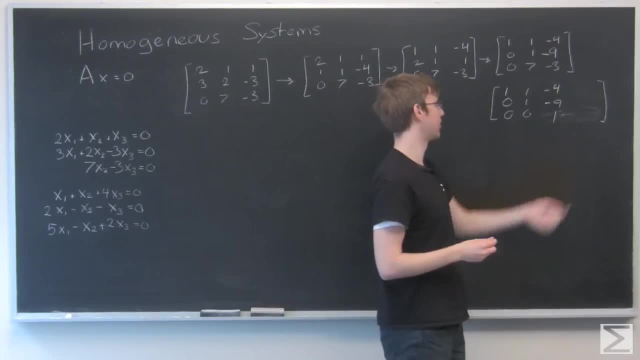 So again, that'll just be some big number which I'll then divide by itself, and that'll be a 1.. And because I have a 1 here now, I can just subtract that out or add that to that 9 times. 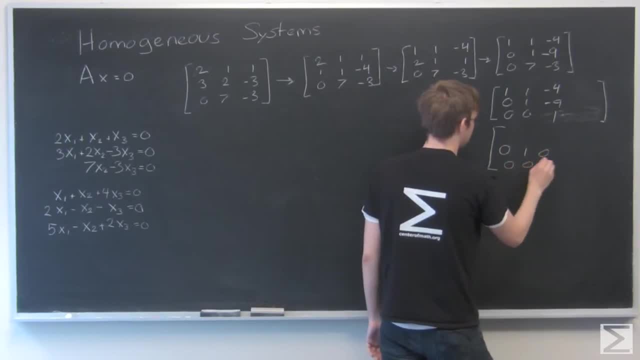 and so in that row I'm going to get 0, 1, 0.. And now I can just subtract from this row, subtract this row from this row. 1 minus 1 is 0, minus 4 minus 0 is minus 4, but then I can do the same with this row and I'm just 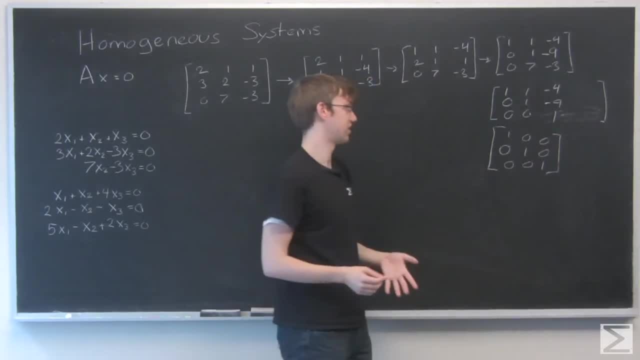 going to end up with that- The identity matrix where I have 1,, 1,, 1.. This is what is called The trivial solution, Because here I have- If you remember, I eliminated my vector of answers because I don't need them- but this: 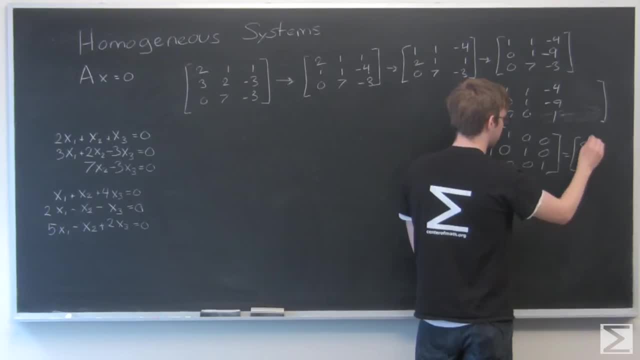 is all equal to that- 0, 0, 0, where we have the x's right there. So what that says is x1 equals 0,, x2 equals 0, and x3 equals 0. And that's the only solution. 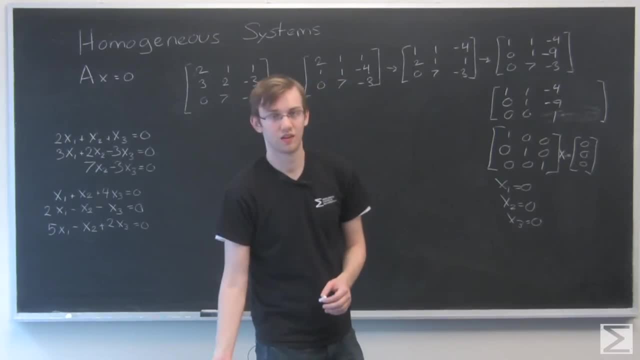 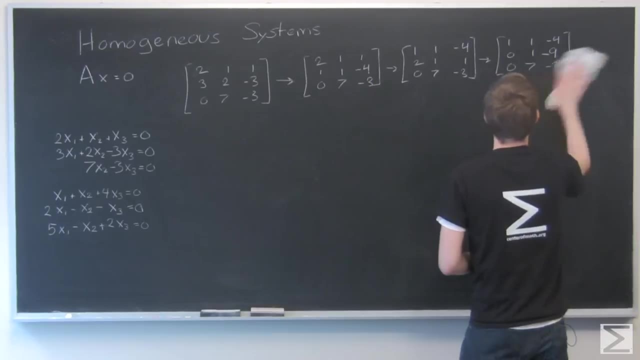 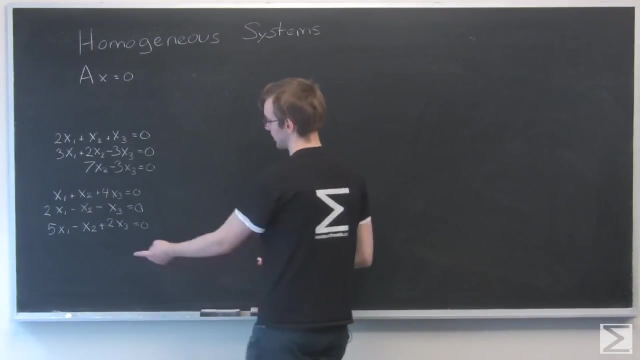 The trivial solution, Where all of my variables are equal to 0.. Now what does an example look like that has more than the trivial solution? Let's write this one as a matrix. I have 1,, 1,, 4.. 2, minus 1, minus 1.. 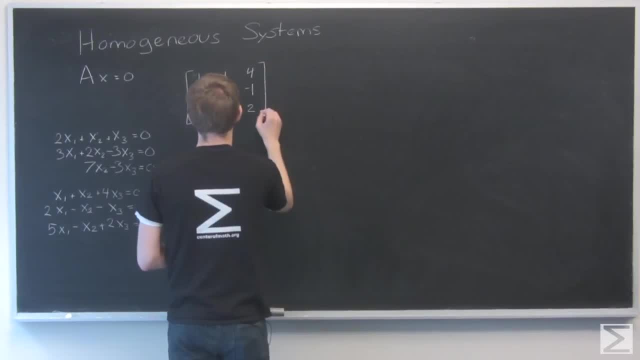 5, minus 1, minus 2.. And again, I don't have to write those zeros because they don't change. I just have to remember that they're there. OK, I'm going to go row 2 minus 2 times row 1.. 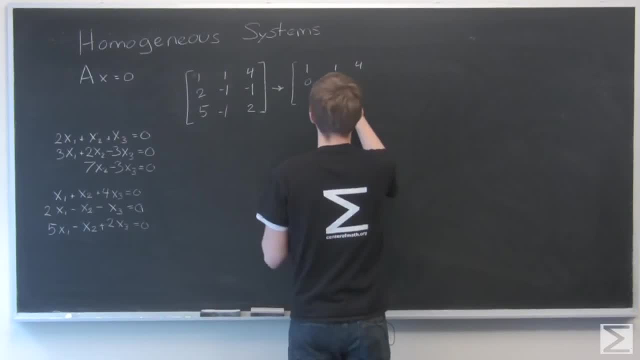 Minus 1, minus 2 times 1, that's minus 3.. Minus 1, minus 2 times 4, that's minus 1, minus 8.. Minus 9.. And I'm going to go this row minus 5 times this row, so that'll be 0.. 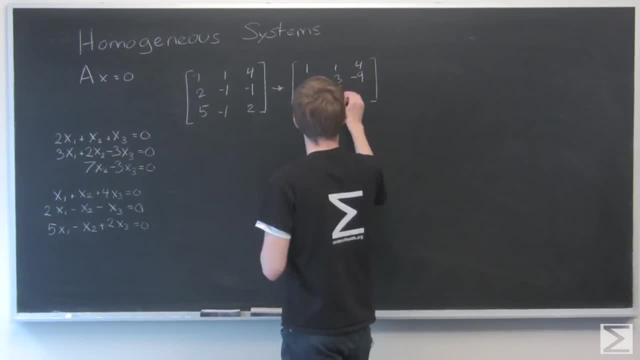 Minus 1, minus 5 times 1,, that's minus 6.. And 2, minus 5 times 4,, that's 2 minus 20,, that is minus 18.. I'm going to divide this row by negative 3.. 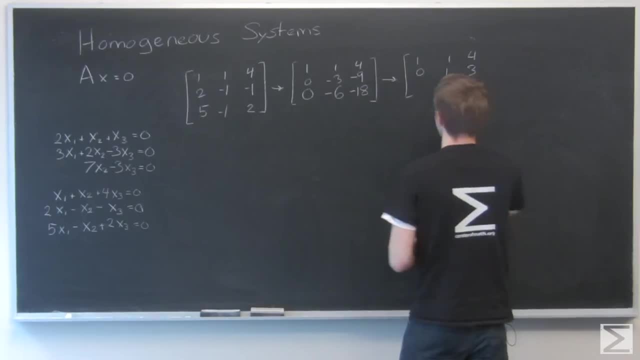 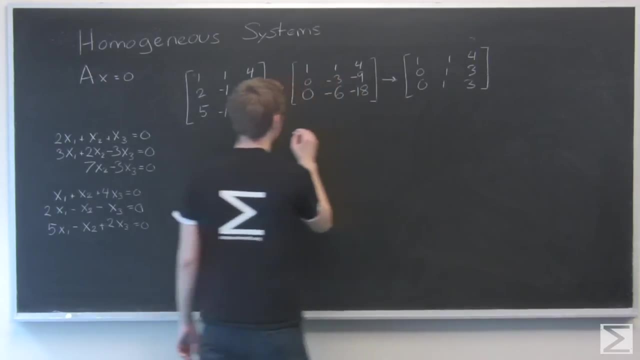 Get 0, 1, 3.. I'm going to divide this row by negative 6, and get 0, 1, 3.. Cool, I can subtract out that row completely. Now I'm going to take the first row minus the second row. 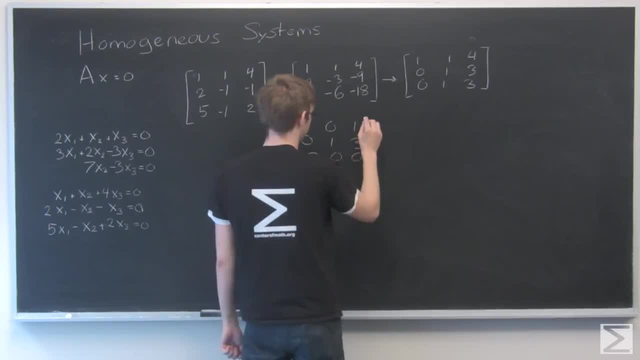 1 minus 1 is 0.. Minus 3 is 1.. OK, So we are here in row echelon form, reduced row echelon form, And x3 is going to be my free variable. I'm going to call that t.